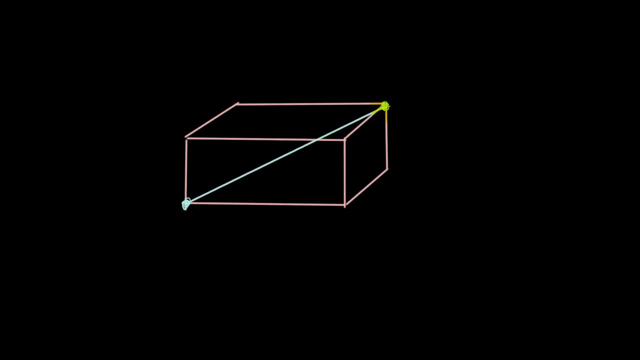 2D, it's 3D, so straight line. So I'm going to draw a straight line from the bottom left hand corner, straight line across that. So how would I find the length of this line, given that, let's say, the bottom horizontal line is 10 centimeters and going across the y-axis, let's say it's 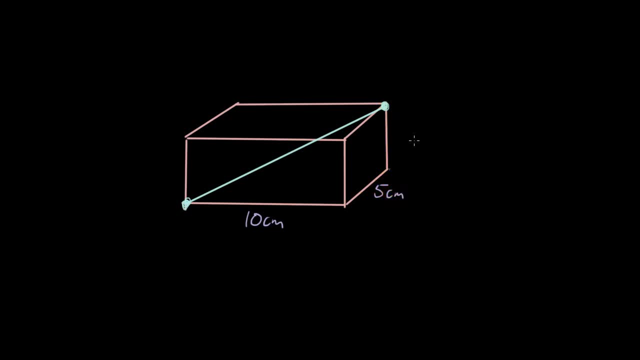 5 centimeters and going upwards, let's say, is 7 centimeters. How do we find this green line? So what I'm going to do is I'm going to show you how to do it the long way, and then I'm going to show you a shorter way. So the longer way is we're basically going to draw, turn this. 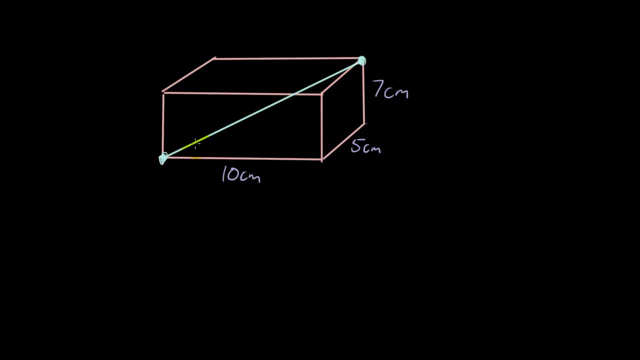 line into a plane. So we're going to turn this line into a plane by drawing from this corner to the bottom corner, to the top right corner and then, during this line, upwards, so we can see a triangle. Okay, so if I just draw this triangle out, isolate the triangle, you can see that this blue line is. 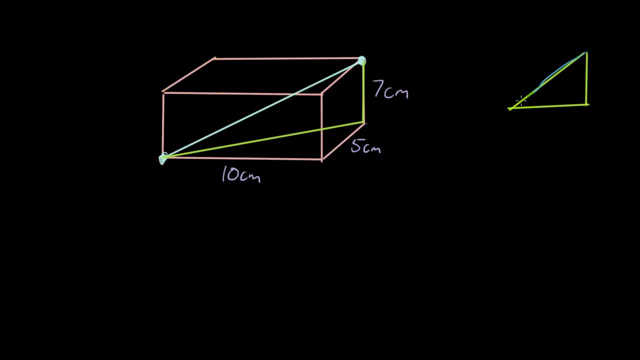 what we're trying to find. so this line is the blue line. This is what we're trying to find. we have the green line. this one going up is seven centimeters, but we have no idea how long this line is, so let's call this blue line y and let's call this. 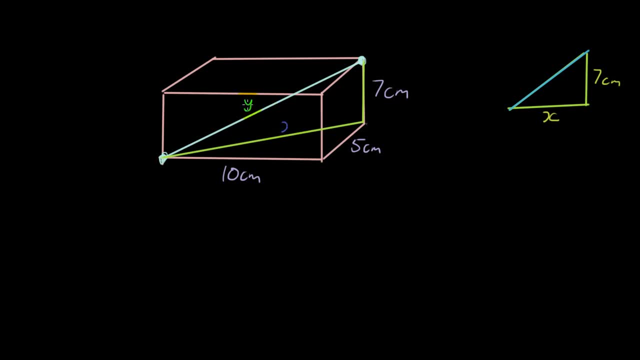 bottom horizontal line. let's call that x and x is. x is what we're trying to find. okay, so we're trying to find x and that's y there. so we want to find y based on pythagoras. so y squared equals 7 squared plus x squared. but we have no idea what x is right now. so how do? 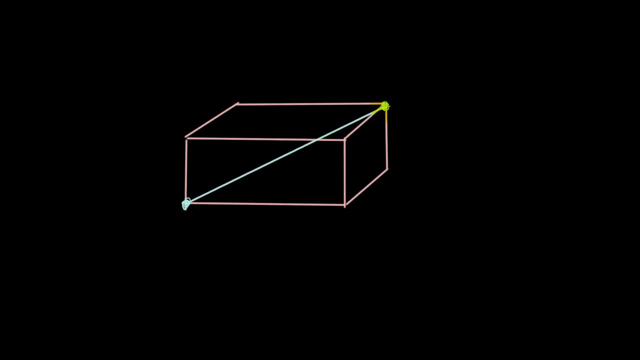 2D, it's 3D, so straight line. So I'm going to draw a straight line from the bottom left hand corner, straight line across that. So how would I find the length of this line, given that, let's say, the bottom horizontal line is 10 centimeters and going across the y-axis, let's say it's 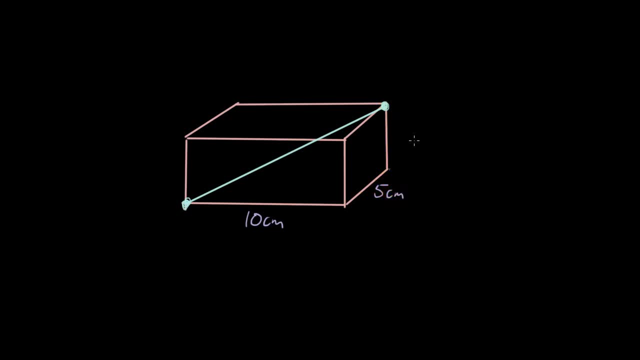 5 centimeters and going upwards, let's say, is 7 centimeters. How do we find this green line? So what I'm going to do is I'm going to show you how to do it the long way, and then I'm going to show you a shorter way. So the longer way is we're basically going to draw, turn this. 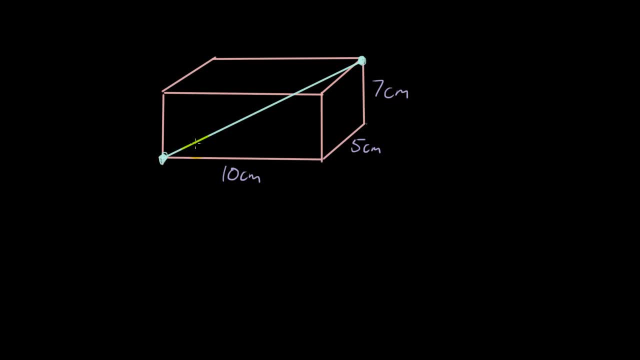 line into a plane. So we're going to turn this line into a plane by drawing from this corner to the bottom corner, to the top right corner, and then drawing this line upwards so we can see a triangle. Okay, so if I just draw this triangle out, isolate the triangle, you can see that this blue line is what we're. 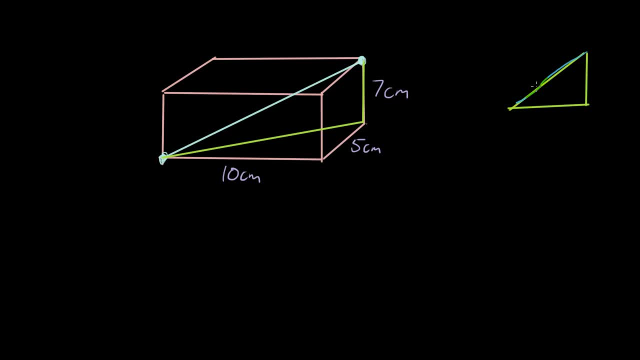 trying to find. So this line is the blue line. This is what we're trying to find. we have the green line. this one going up is seven centimeters, but we have no idea how long this line is. so let's call this blue line y and let's call this. 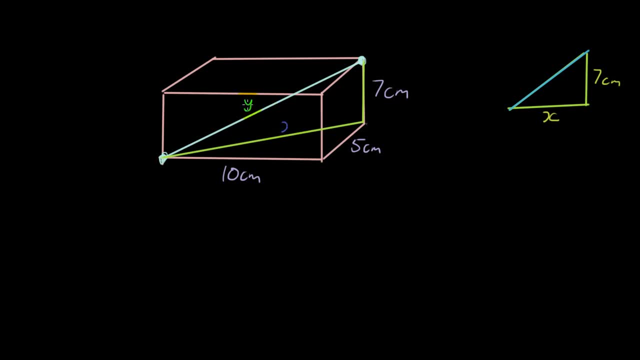 bottom horizontal line. let's call that x and x is. x is what we're trying to find. okay, so we're trying to find x and that's y there. so we want to find y based on pythagoras. so y squared equals 7 squared plus x squared. but we have no idea what x is right now. so how do?